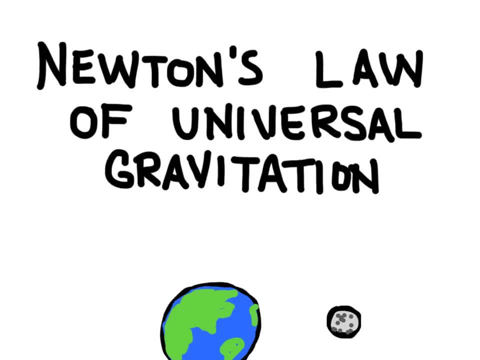 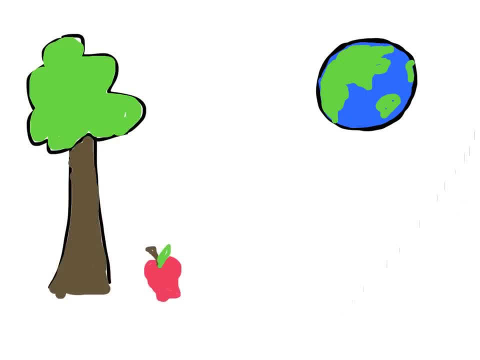 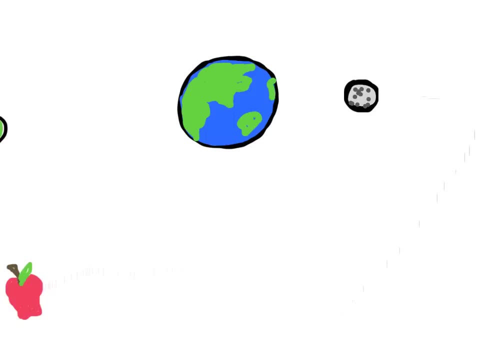 In this video, we're going to talk about Newton's Law of Universal Gravitation. Now, as the legend goes, Isaac Newton saw an apple fall from a tree, And it's thought that he began thinking. does that same force that caused the apple to fall towards, or be attracted to the earth? 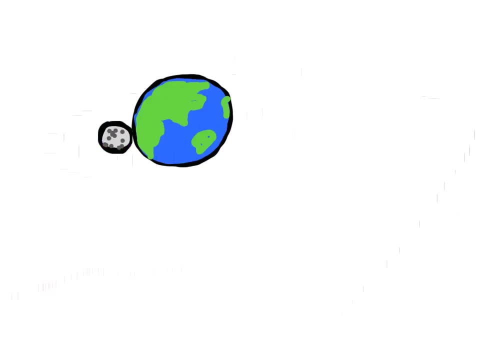 cause the moon to be attracted to the earth and stay in orbit. So this was what his thinking was, and he investigated this and he found two things. First of all, he found that the force of gravity was proportional to the distance between the two objects. 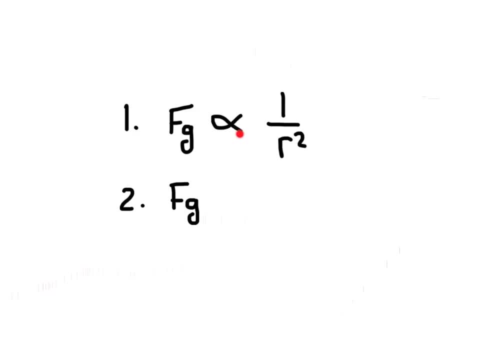 And, more specifically, he said that the force of gravity is proportional to the inverse square of the distance between the object. This is what r represents: the distance between the centers of the two objects. If you're not familiar with this symbol, that means proportional to. 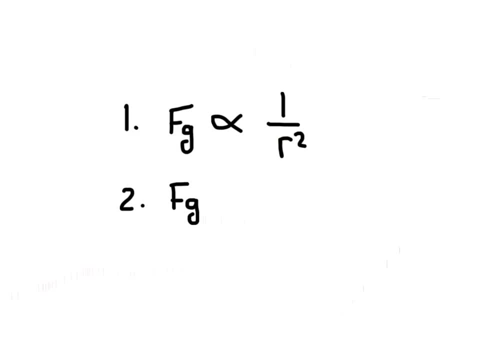 In other words, they will change at the same rate. They're not equal to each other, they change at the same rate. The other thing that he found is that the force of gravity is also proportional to the size of the objects, or in other words, their mass. 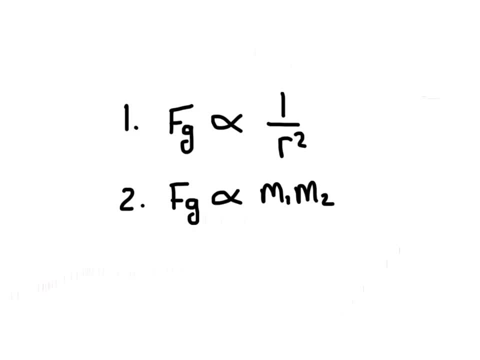 So we have the mass of the first object times the mass of the second object. Now these two things go together to form this equation right here. So we have our masses on top over the distance squared, And we had to add this thing in here. it's called the universal gravitational constant. 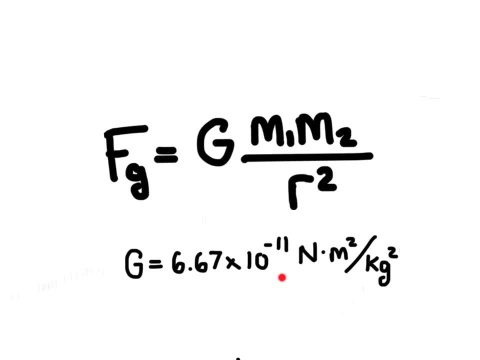 Newton didn't discover this number right here, but this is what that constant is equal to. So G, this capital G, is just a substitute in this number with these units. Newton didn't discover this. this was discovered much later, in the late 1700s, by a scientist named Henry Cavendish. 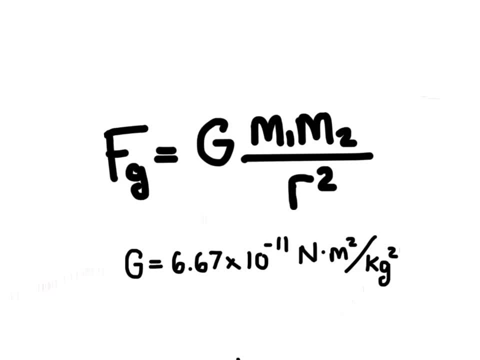 Now we won't get into his experiment, but basically he was able to determine pretty accurately the force of gravity between two objects of known mass and knew the distance between them, And he was able to solve for This value and he determined it to be this right here. 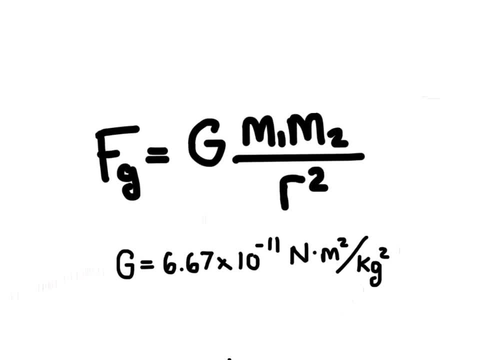 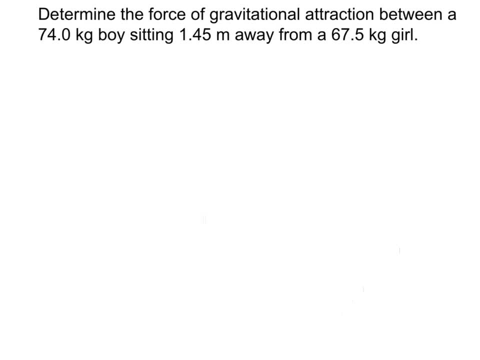 So we need that to solve any question involving gravitation between two objects. So here's an example of a question that's going to involve solving for the gravitational force. We'll read this one and then we'll solve this one together. It says: determine the force of gravitational attraction between a 74 kilogram boy sitting 1.45 meters away.